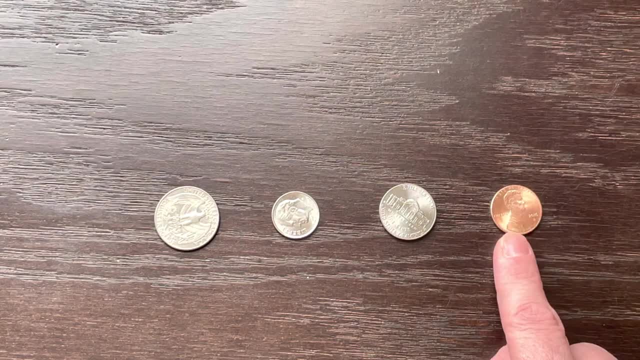 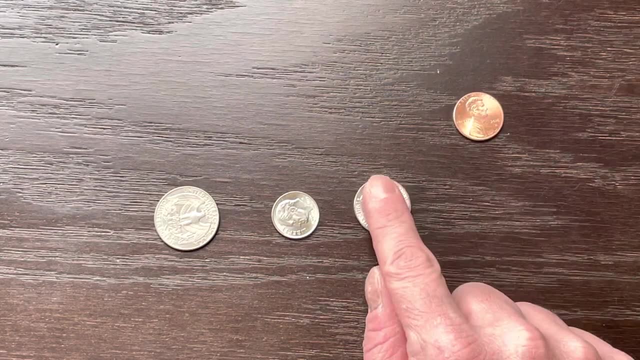 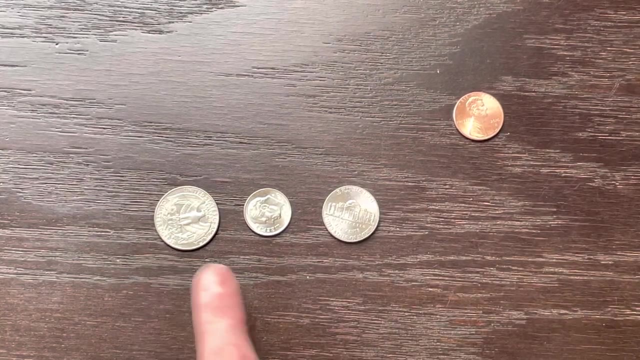 Penny, penny, easily spent, Copper, brown and worth one cent. So pennies are brown. So those are the easiest ones to identify because of their color, and pennies are only worth one cent. Now these three can be a little trickier because they are all silver and they do look similar, but there 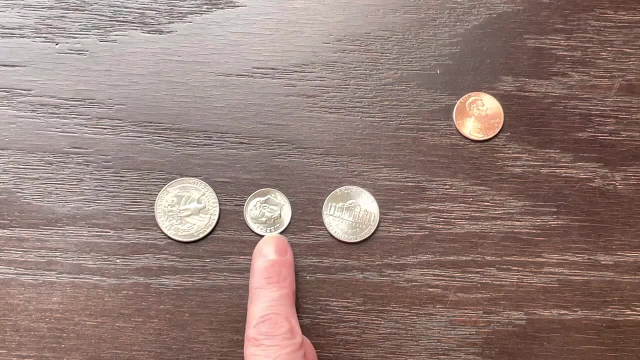 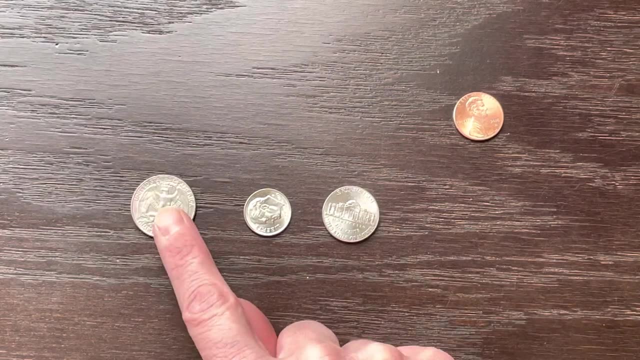 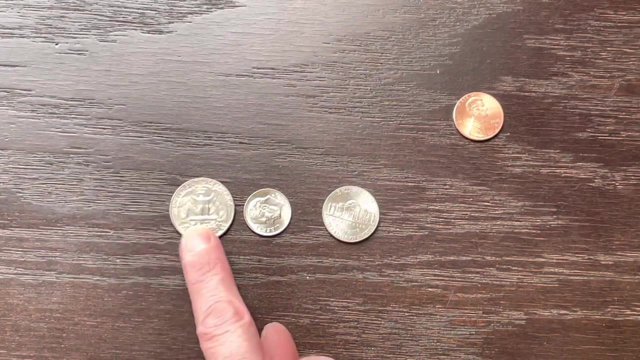 are differences about them. One thing is you can use size to help you identify them. So the biggest coin in these four is a quarter, Quarter, quarter. big and bold. You're worth 25, I'm told. So if you look at these four, you can see that they're all silver. So you can see that they're all silver. 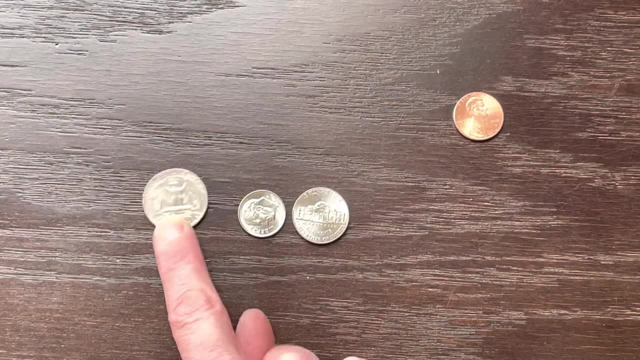 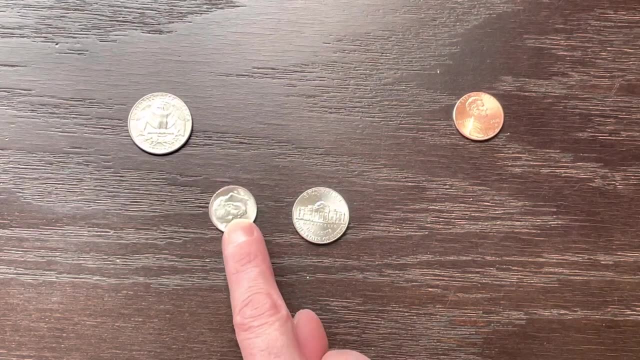 So if you look at these four, you can see that they're all silver. So if you look at these four, you can see that the quarter is the biggest one, And so if you can find the biggest one, you can see that is a quarter. Same thing with the dime: If you look closely it's the smallest one. 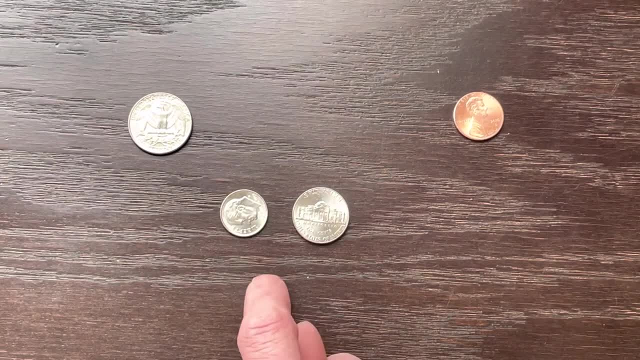 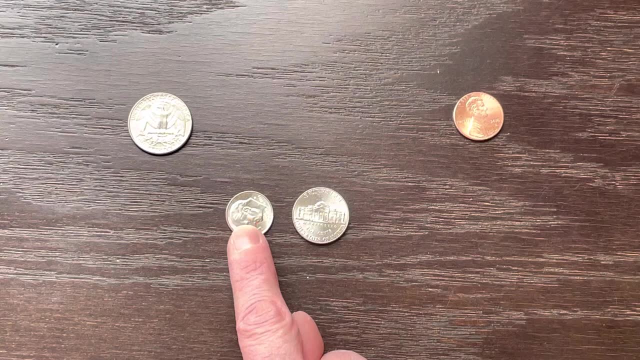 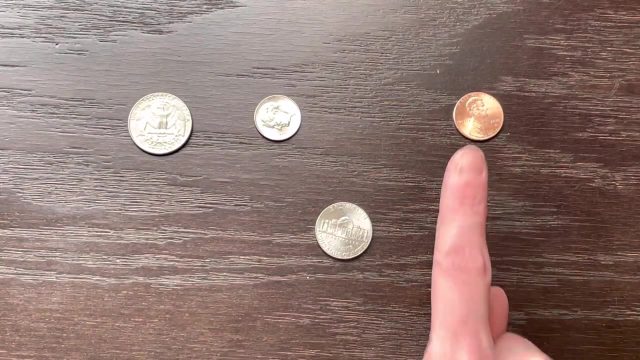 So you can find the dime by looking for the smallest silver coin: Dime, dime, little and thin. I remember you're worth 10.. Now, nickel is probably the trickiest one to identify because it's not the. But one thing that is special about a nickel is it's the only silver coin of these three. 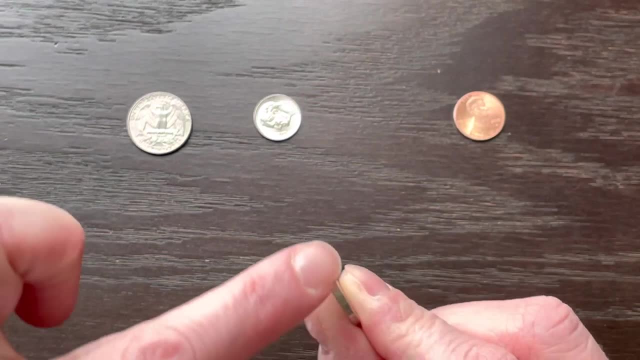 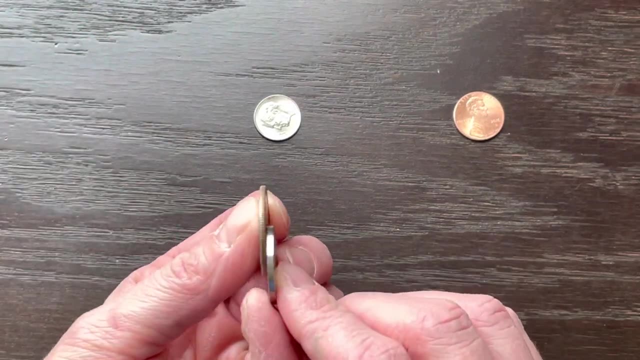 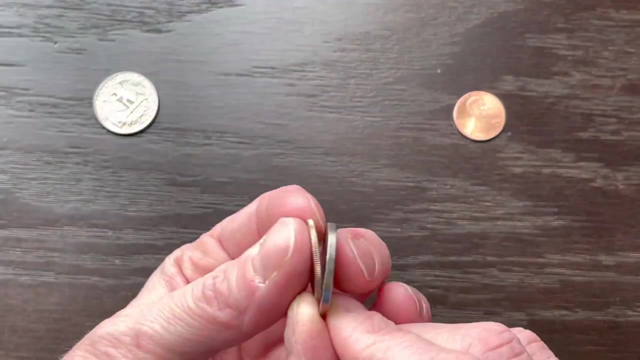 that has smooth edges. So if you take your finger and rub your finger on the edge, it's smooth, It doesn't have any bumps. And if you look at the edge of a quarter you will see it has little bumps on it. So it's rough on the side of a quarter and it's also rough on the side of a 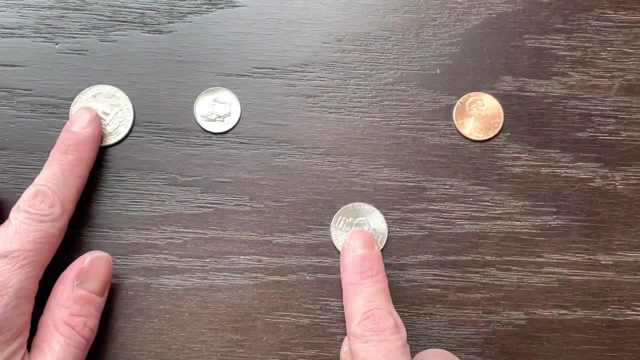 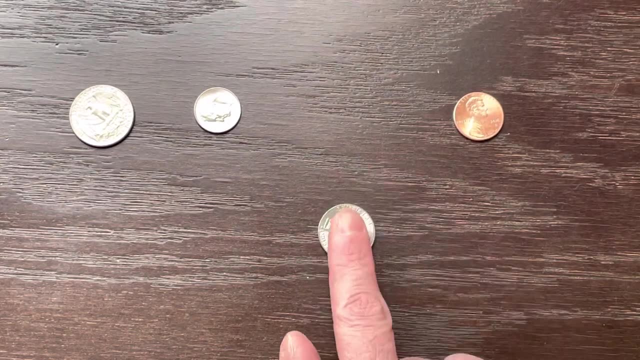 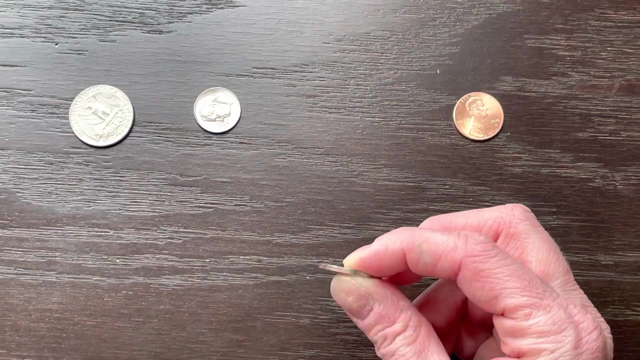 dime, It has those little lines. So nickel, nickel, thick and fat, You're worth five cents. I know that The reason we say thick and fat is because it is the thickest coin as well. It's the thickest diameter going across this way thickness. But I think the 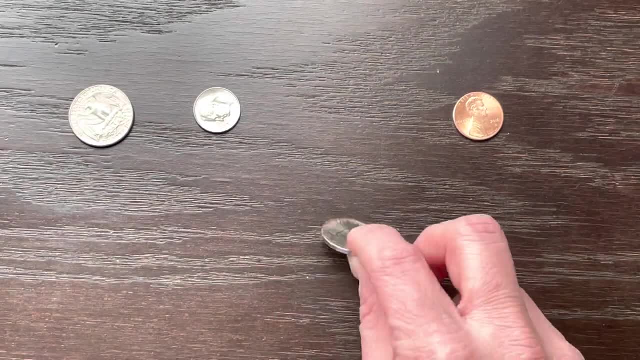 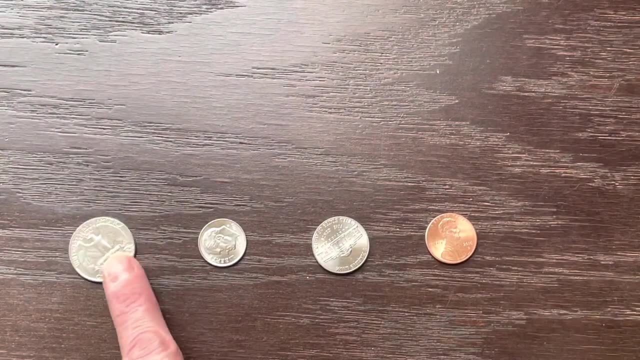 easiest way to identify is just by touching the edge and feeling that smooth edge. Smooth edge means it's a nickel. So one more time we have: penny is brown, quarter is the biggest, dime is smallest and nickel is the middle sized one with the smooth edge. So if you look closely you can. see that it has smooth edges. Have a great day, little sprouts.